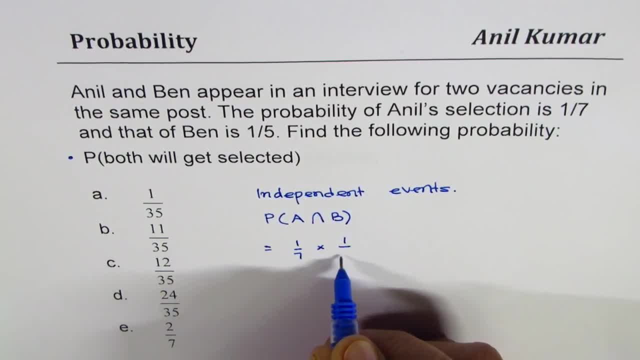 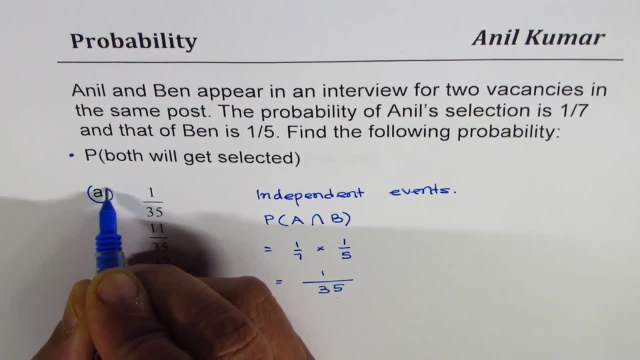 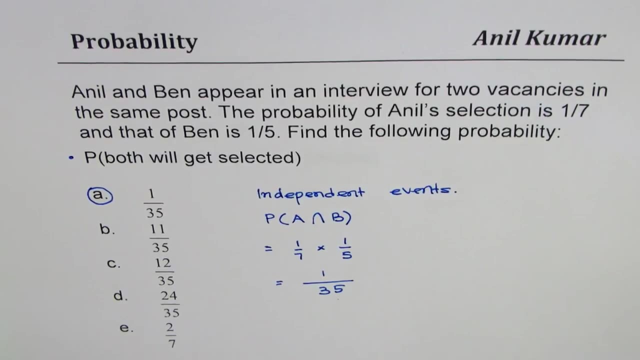 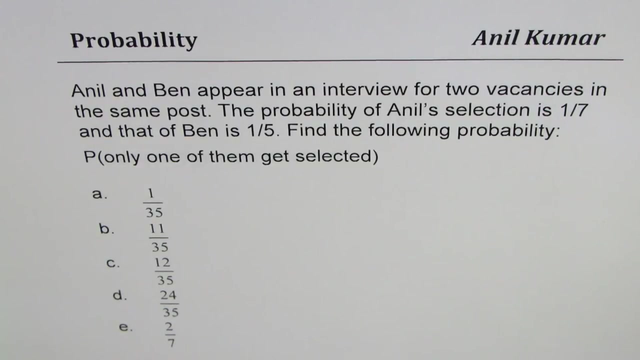 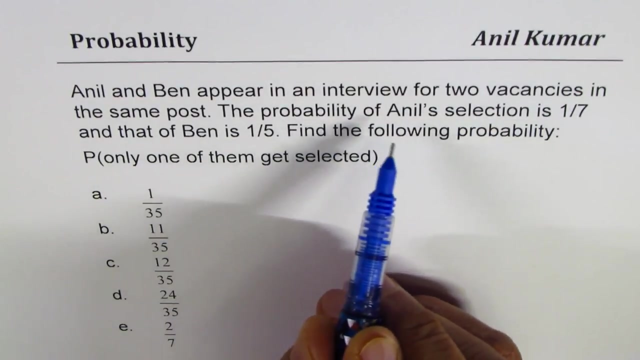 So it is 1 out of 7 times 1 out of 5. And what we get here is 1 out of 35. And so A is the correct choice right Now. if we change the situation a bit, we'll get to the next question, which is, scenario being the same, that Anil and Ben appear for an interview for two vacancies, where probability of Anil's selection is 1 out of 7 and that of Ben is 1 out of 5.. 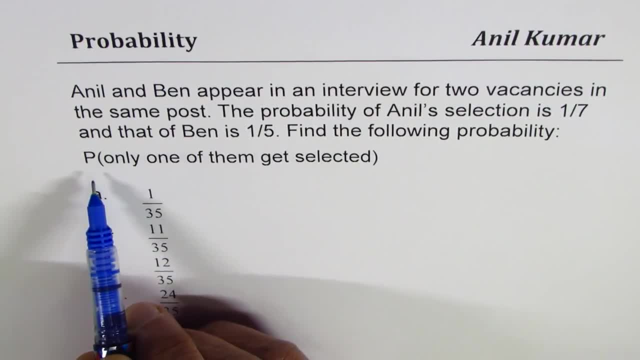 And this time we'll find probability of both of them getting selected. We'll find probability of only one of them get selected. right, Only one of them get selected. The choices are again the same: 1 out of 35, 11 over 35, 12 over 35, 24 over 35 and 2 out of 7.. 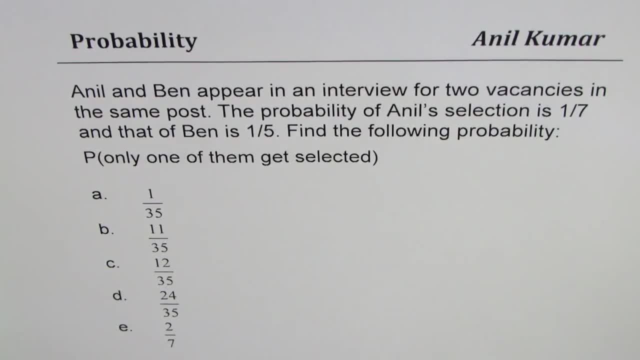 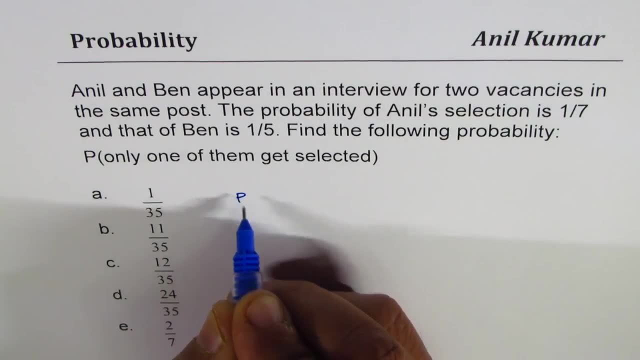 What do you think is the right choice and why? Now, when we say that only one of them get selected, it really means that we are looking for probability of A getting selected and not B. So A gets selected and not B means B prime. that means: 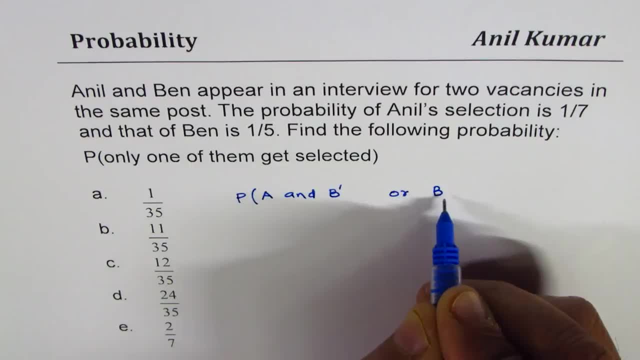 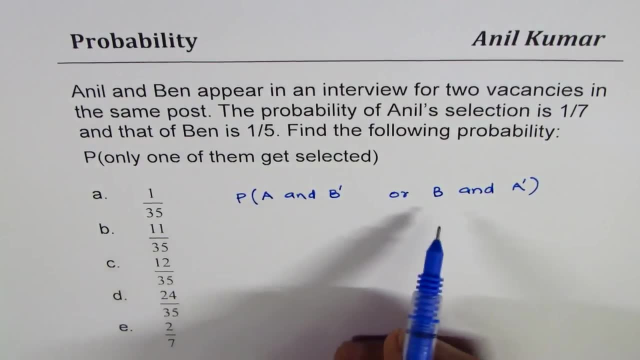 not B, or probability of B getting selected and not A right. So that is how you can see: that only one of them will get selected. So that really means we are talking about probability of A and means you have to multiply probability of not B, or means you have to add. 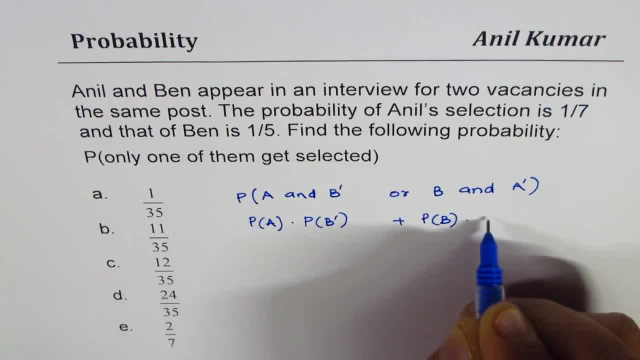 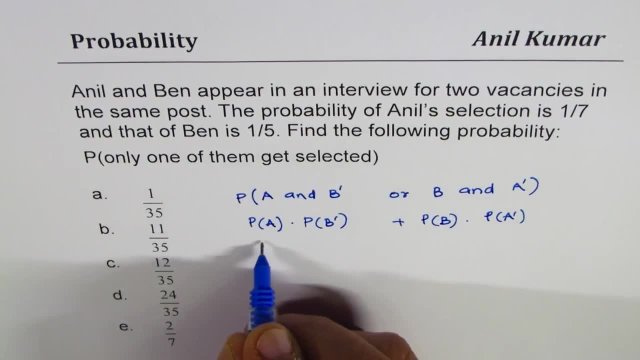 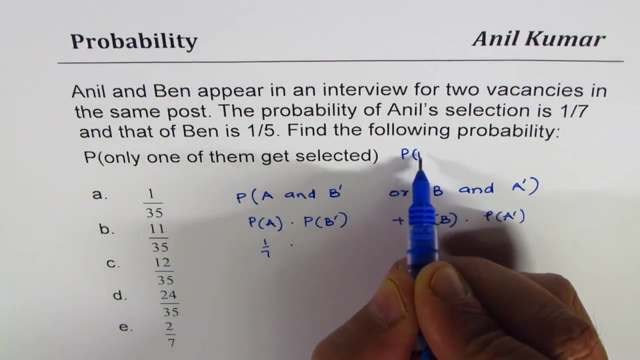 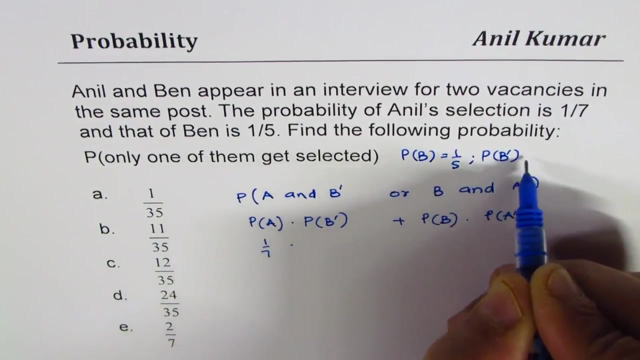 probability of B and probability of not A. correct Now. probability of A is 1 out of 7.. Probability of not B: when we know the situation, when we say probability of B is 1 out of 5, then probability of not B is: 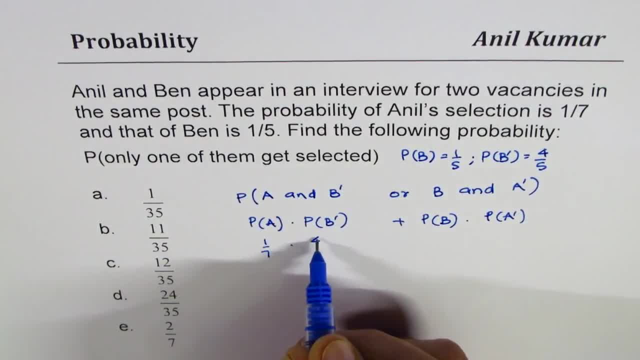 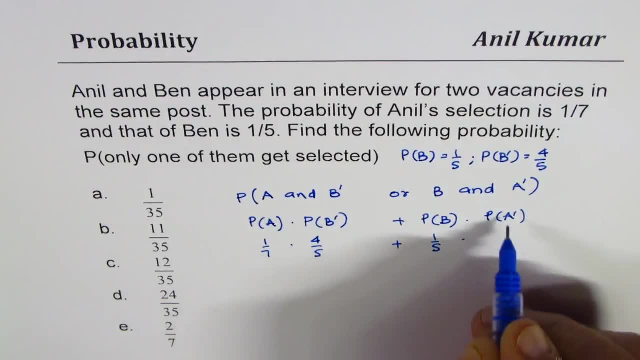 4 out of 5, correct. So that is 4 out of 5, plus probability of B is 1 out of 5 and probability of not A will be 6 out of 7. correct, 6 out of 7.. Since 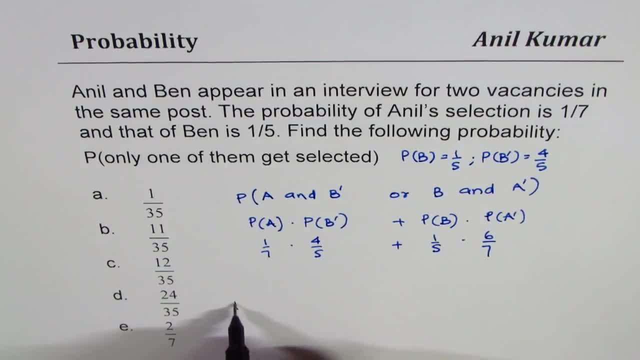 we know that. let me write down here: probability of A is 1 out of 7. that means probability of not A means 6 out of 7, right? You could always find this as 1 minus 1 out of 7. is that ok, because total probability is 1, right? 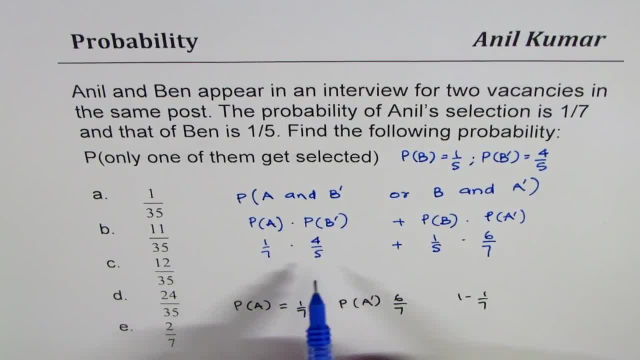 So you get that combination and when you add this up, you get your result. this is: when you multiply this, you get 4 out of 35 plus 6 out of 35. that gives you 10 out of 35, and you can simplify this. dividing both by 5, you get 2 out of 7. is 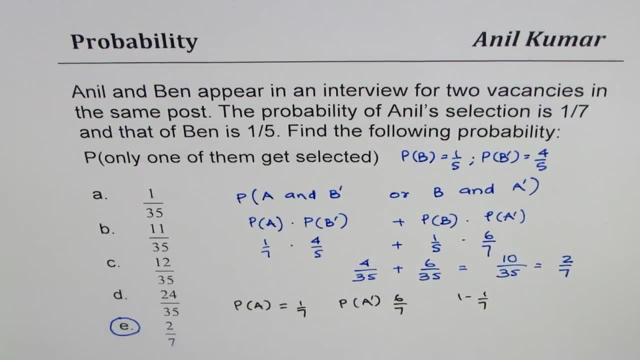 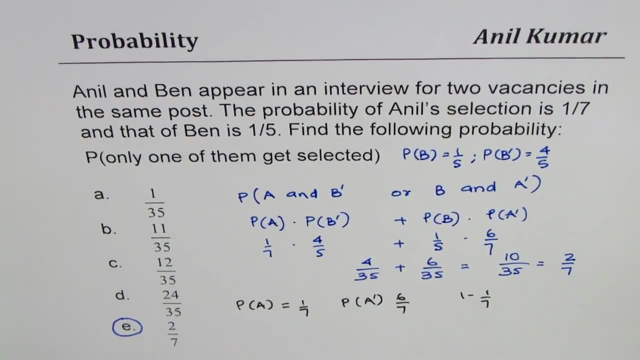 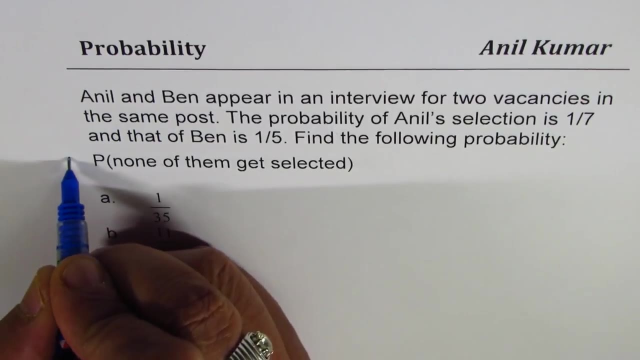 it. okay. so the option is E, which is 2 out of 7. so only one of them get selected, the probability is 2 out of 7, and now we have changed the question a bit more. let's say, part C of this question is: let's write on this as third part of this question, conditions being same. 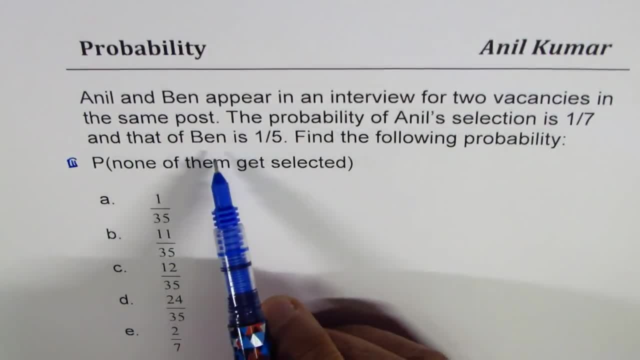 probability of Anil getting selected is one out of seven. probability of Ben getting selected is one out of five and there are two vacancies. now we need to find the probability that none of them get selected right now of them gets selected. So that is the probability which we need to find and that really means we are trying. 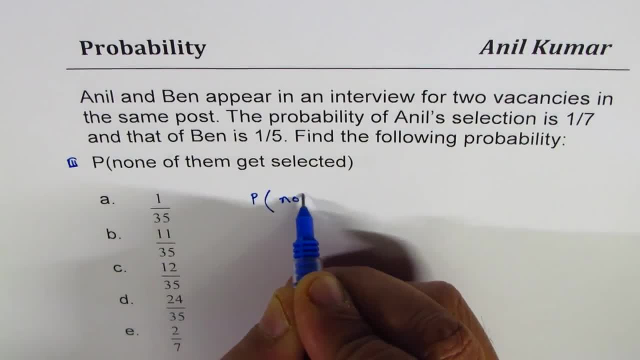 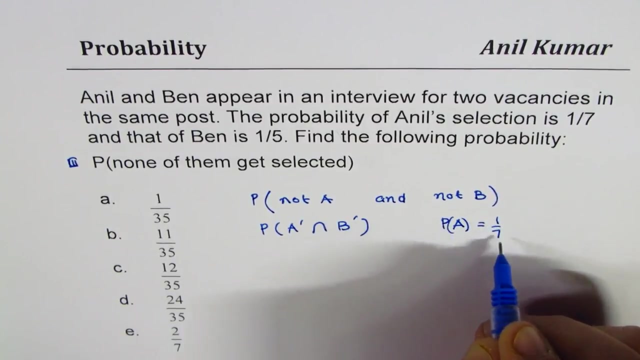 to find probability of not A and not B correct. not A or not B, that means probability of A prime and means intersection, right So, and means intersection of B prime. Now we, when we say probability of A is 1 out of 7, that means probability of not A means 6 out of. 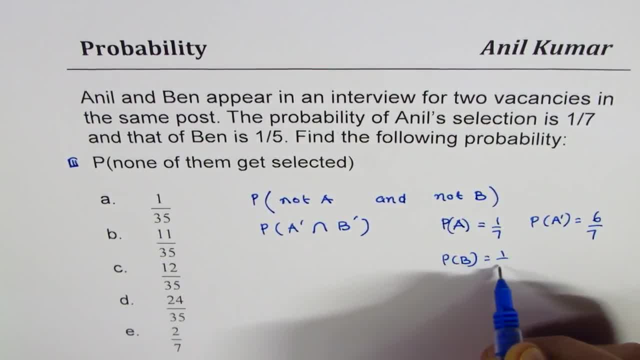 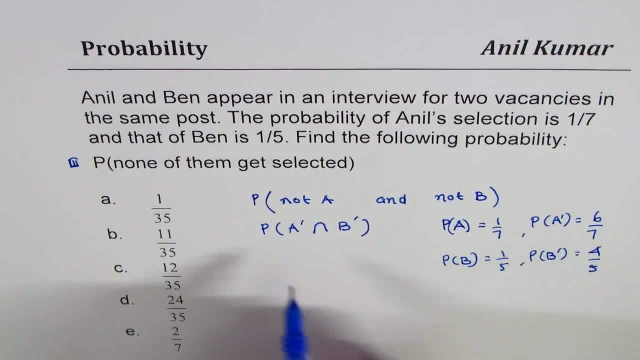 7. When we say probability of B is 1 out of 5, we know probability of not B is 4 out of 5, correct? So here we can just multiply these and get the result. So it is 6 out of 7 times. 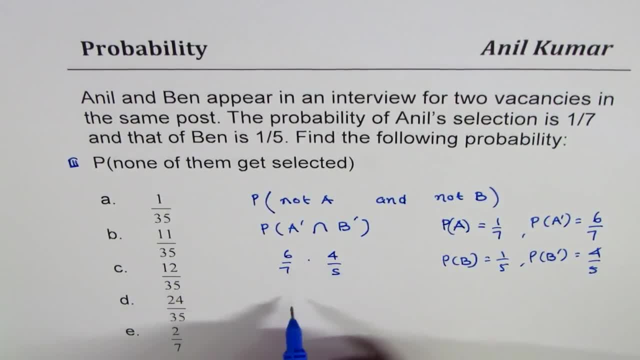 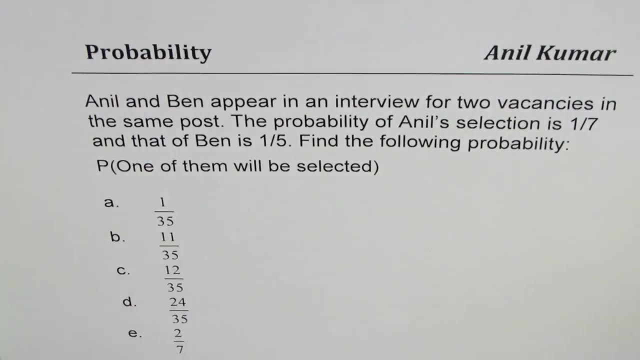 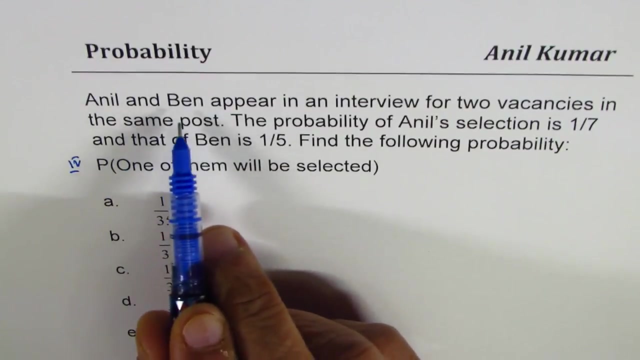 4 out of 5.. and that gives you 24 over 35, correct? So option D is the right option. So let us look into one more condition in the same scenario. Let us call this as the option 4.. Anil and Ben. 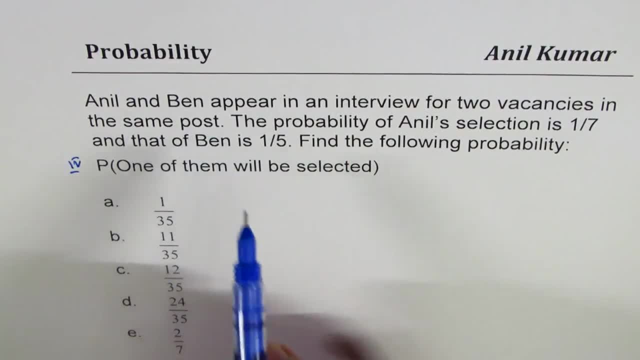 appear in an interview for two vacancies in the same post. Probability of Anil's selection is 1 out of 7 and the probability of Anil's selection is 1 out of 7.. So the probability of Anil's selection is 1 out of 7. that is what we will do. is somebody wants to down that it will. 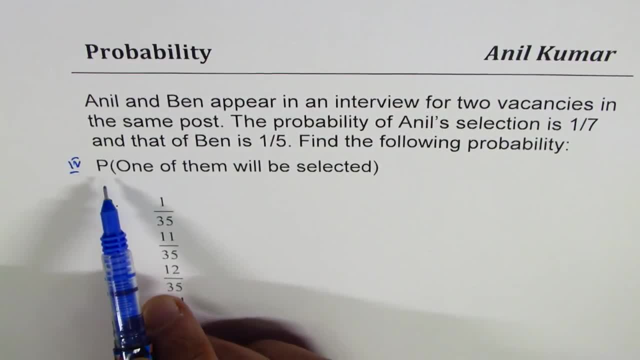 say is that Ben had chosen. Ben has chosen, So 5 cancel the goal. terrace, Danke. This player does not know how to join, So Ben has chosen. Ben has chosen. If I record that winners or the other players has chosen, it is 2, so so 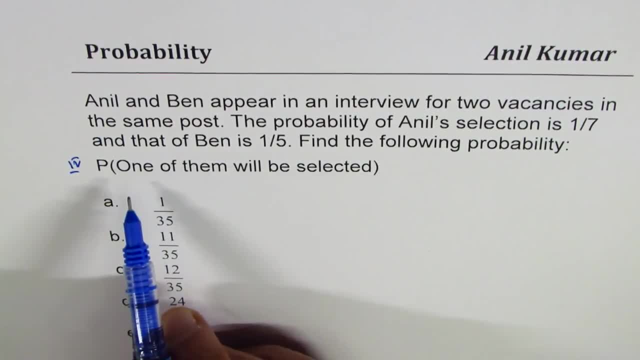 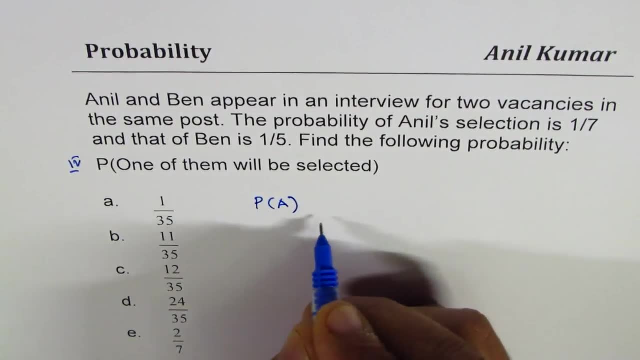 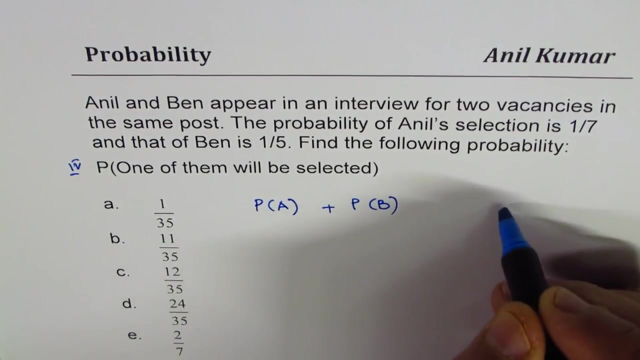 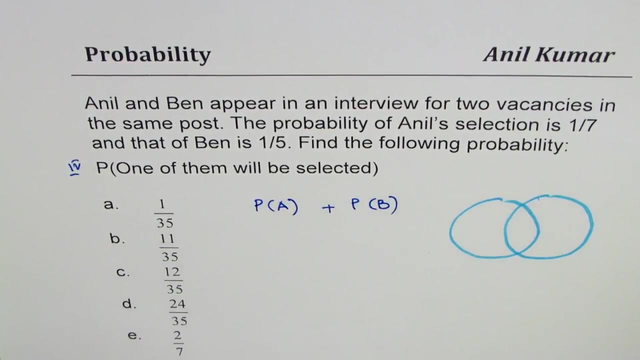 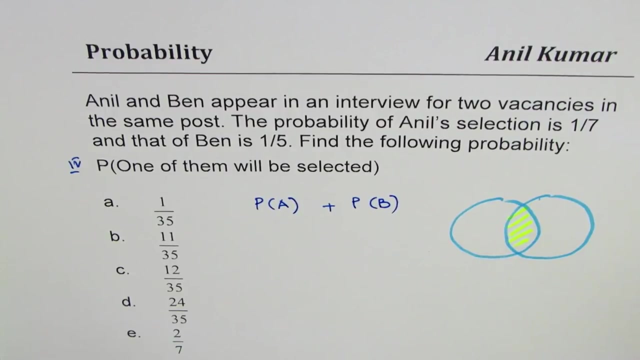 You can see the scenario. It's kind of like this: Let's say, probability of Anil and Ben, There is always an overlap that is both getting selected. So when we count it, we count this overlap twice and therefore we should take out probability of both will get selected. 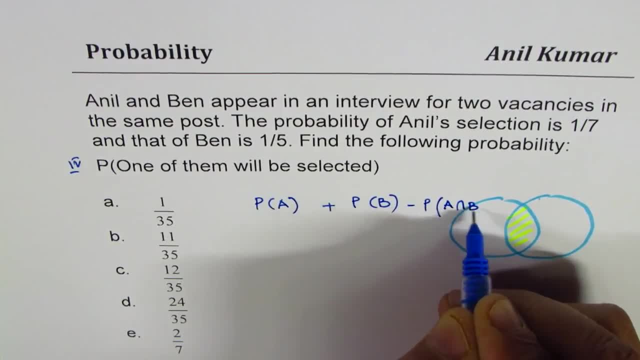 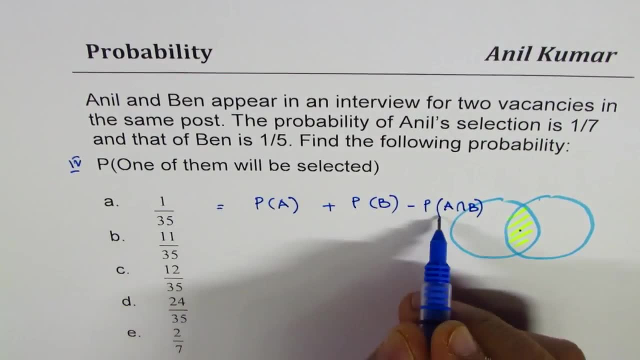 So probability of A and B getting selected, because we counted this twice, the intersection between them. So this is from principle of inclusion and exclusion. Probability of A is 1 out of 7, plus probability of B is 1 out of 5.. Take away, probability of both is product of these two right, 1 out of 7 times 1 out of 5.. 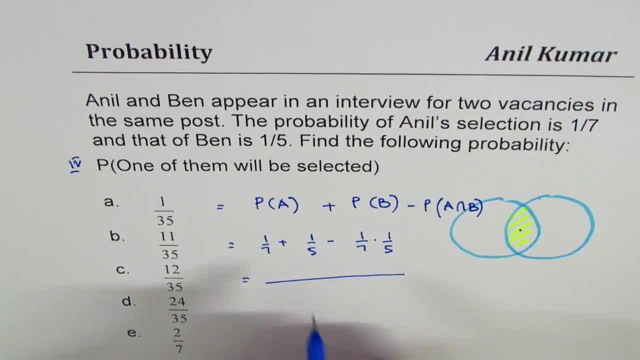 That gives us- We can write, Common denominator is 35.. 5 plus 7 minus 1, and that gives us 5 plus 7, 12 minus 1, 11, 11 out of 35. So it is option B for us. 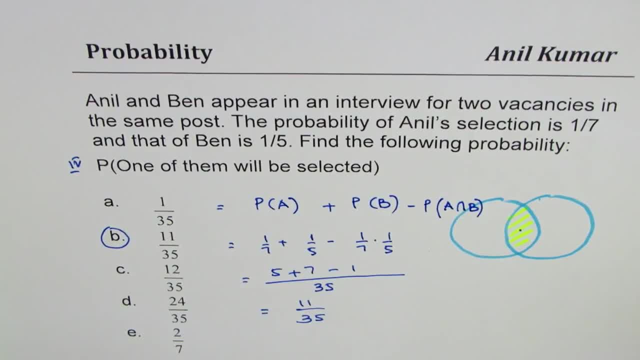 So in this particular video we have learned that if there are two positions with known probabilities, then under different conditions, what could be the probability? So we have considered the case that both of them will be selected. Only one of them get selected.